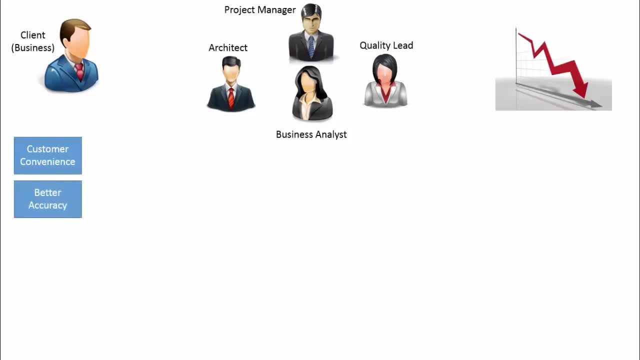 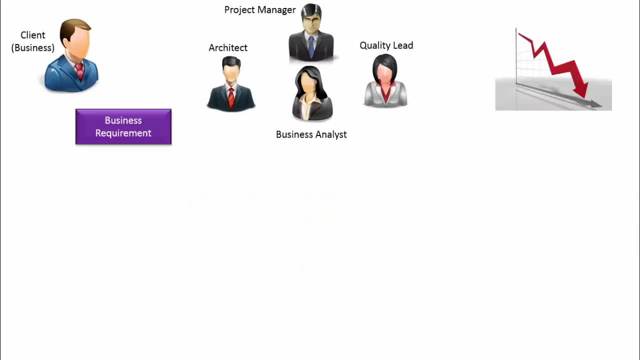 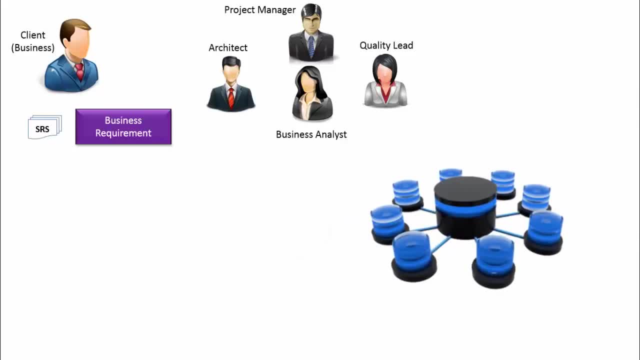 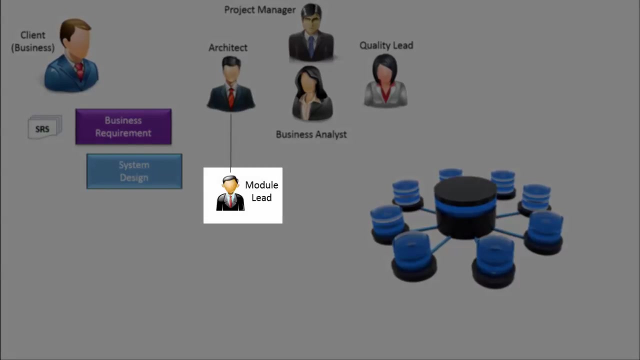 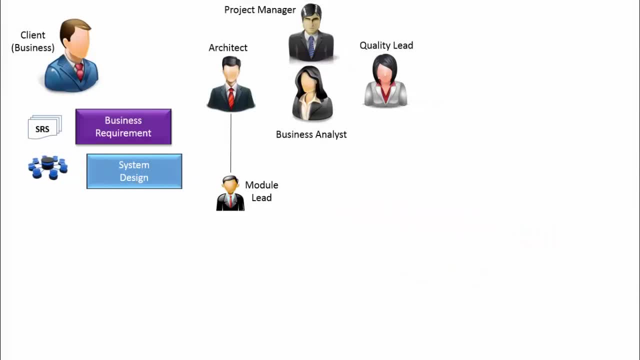 For very large projects there can be a team of architects and they may have a chief architect as well. The system is then analyzed from functionality perspective. For example, multiple pages might be required for the website. Each page would have related functionalities grouped together like one page for showing. 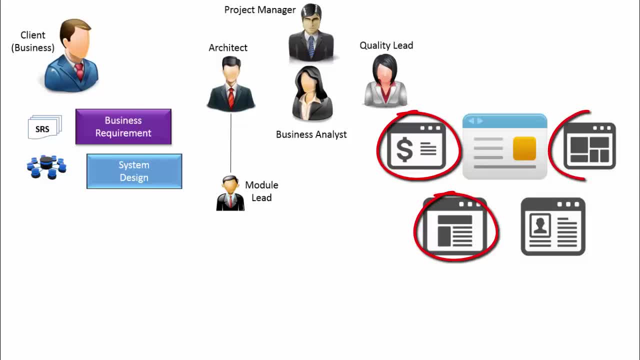 bank balance. second page for fixed deposits, third for bill payments, fourth for user profile and so on. In this case, every page is meant for different but related functionality. These can be called as modules. Now the modules may interact with each other. 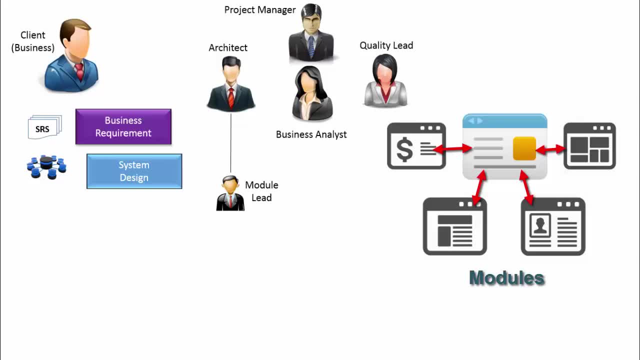 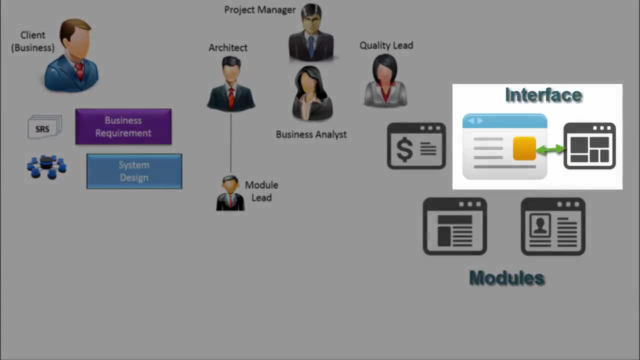 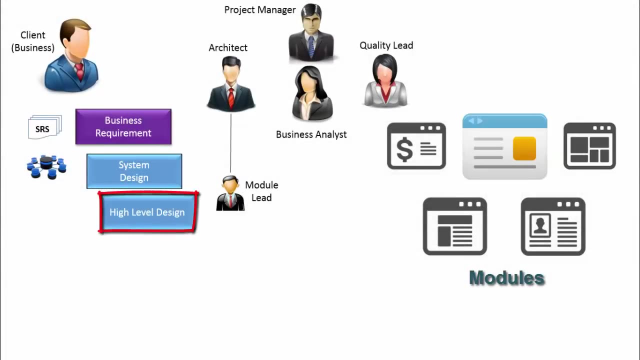 For example, homepage for the website might show summary from each module and contain links to various pages. Identification of high level module and defining their interfaces- that is, how one module is going to interact with other module- is done through high level design. Generally, a group of programmers work together. 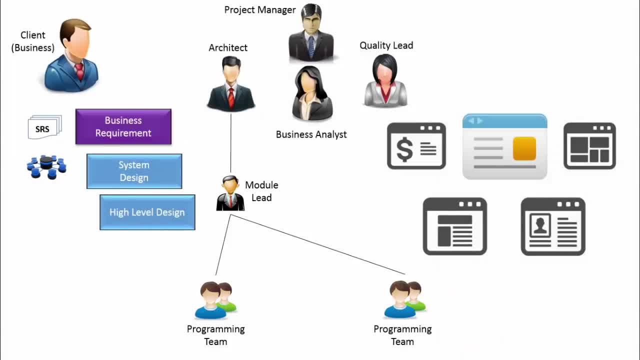 They work on a module led by respective module. lead By the end of this phase, the team comes up with high level design document, or in short, HLD. Every module may consist of smaller units of functionality. For example, a method can represent one unit of functionality. 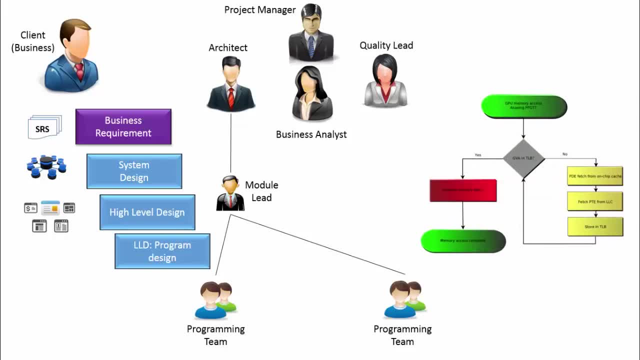 The programmers refer HLD to come up with such units and their algorithm, flow charts, data flow diagram, class diagram, etc. This is called detail design or low level design or LLD. The architect and module leads keep on reviewing the design documents as and when they are produced. 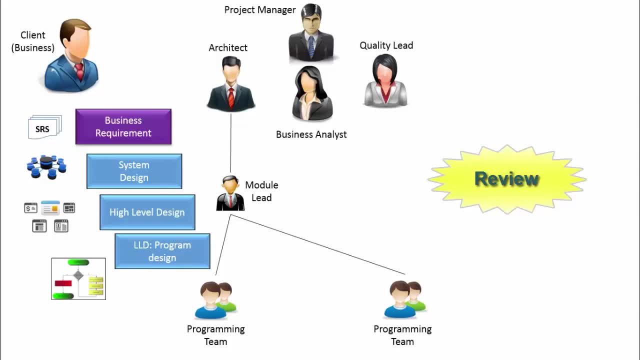 and provide their feedback comments to the authors of those documents. Review happens for every artifact, like SRS, HLD, LLD. These are reviewed by internal or sometimes subject matter experts from outside the team. These review comments are documented and are tracked to see if any of the documents are. 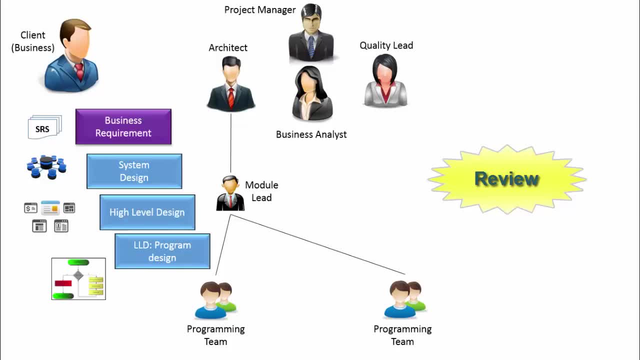 correct If appropriate action is taken for open action items. This is usually done with the help of tracking tools. After the review of LLD, programmers start writing source code for individual units. Programmers then review each other's code to see if the code is written properly. 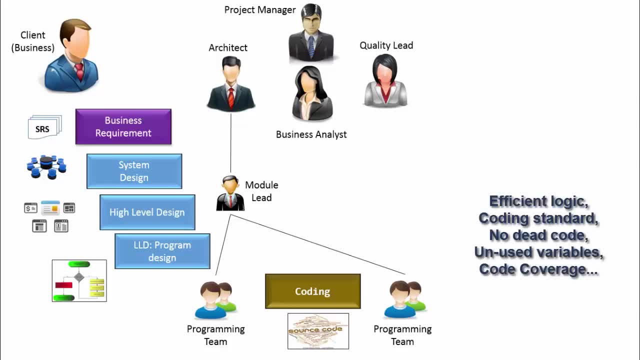 For example, they may check if the code written is efficient and it has followed coding standards and there is no dead code or unused variables etc. This is called peer review. Once a program is written, it is tested for its correctness. This process is called testing. 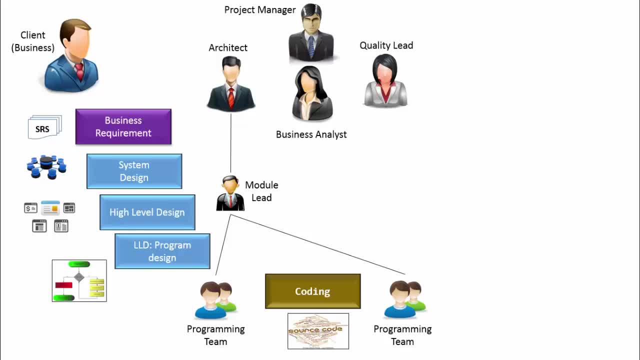 Various types of tests are carried out on the code. The first one is unit testing. Here, individually, the units, like methods and classes, are validated against their LLD. What it means is, by unit testing, programmers verify that the code is structured as per the low level design document. 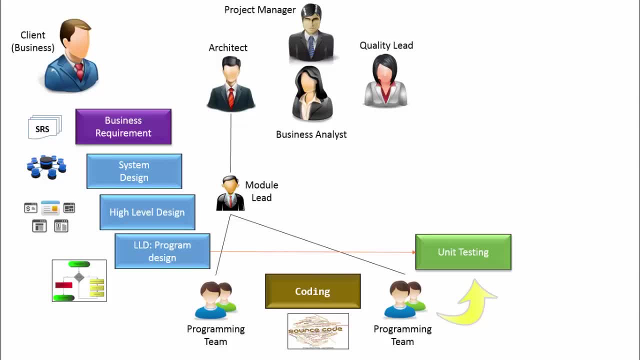 It is carried out by the developers before they hand over the code. It is carried out by the developers before they hand over the code. It is carried out by the developers before they hand over the code. After testing, it is assigned to the testing team for further processing. 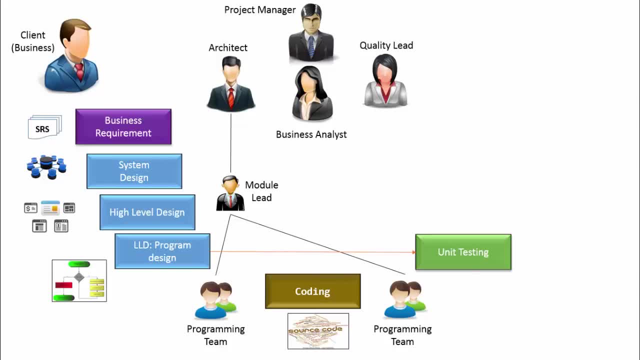 So a unit tested code is an outcome of the coding phase of the software development lifecycle. This code is then further handed over to the testing team, which is led by the quality lead. The individual units may work fine, but they may fail when integrated with other modules. 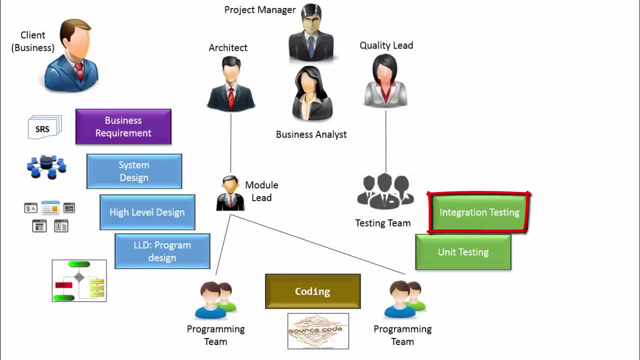 This is checked during integration testing. This type of testing is done to validate if behavior of integrated modules are as per the high level design. On the similar lines, system design is validated during system testing. Various tools are used to check the performance of software. For example, a tool may help. 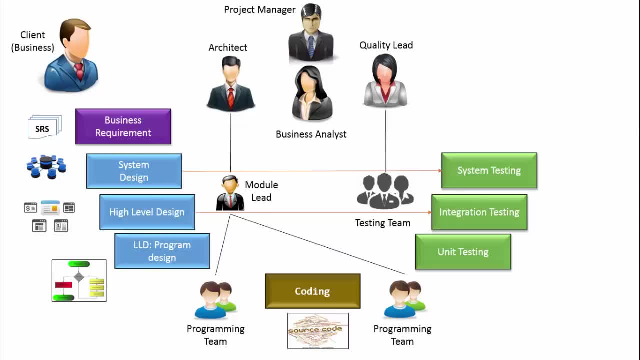 in generating 500 virtual simultaneous user requests to the web server to check the peak load performance of the website. Any non-conformance is logged as defect. What it means is if the software does not behave as per the design expectation, then this is reported as a bug. 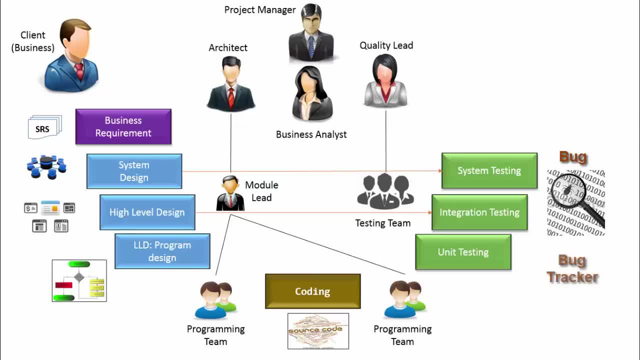 This is again usually done with the help of a software called Bug Tracker. The author of the code then fixes the problem and sends it back to the tester, who will revalidate them. The process keeps on repeating till the problem is fixed. Finally, the software is delivered to the client, who then validates whether the business 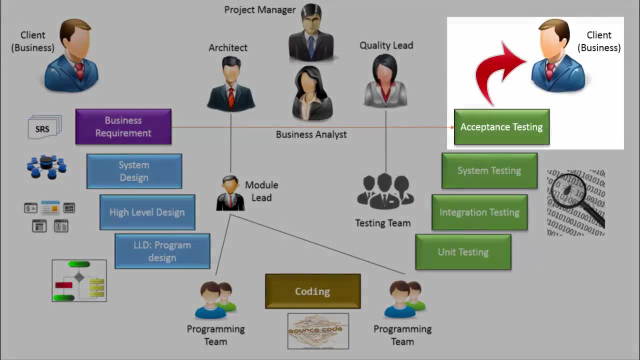 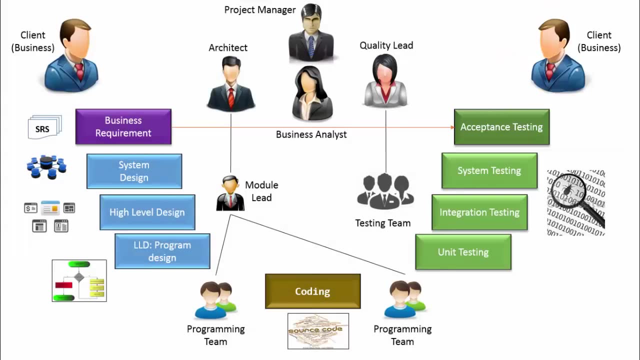 requirements mentioned in the SRS are taken care. This is called User Acceptance Analysis testing, or in short, UAT. After UAT, the software is deployed in the production environment. The entire process model looks like a V structure, so this is also known as V model. 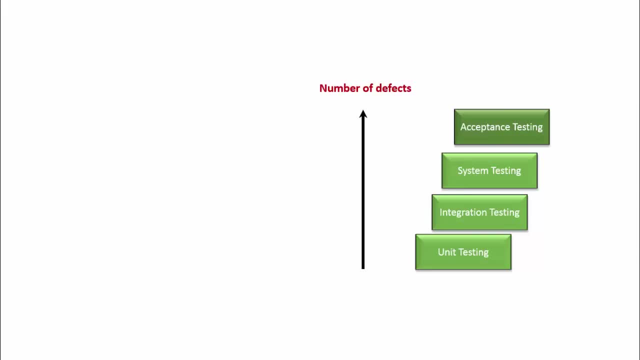 Note that the number of defects identified at the former testing is more than the later. However, the impact of identified bug on cost keeps on increasing as we move from development to production, And when a bug escapes the testing process and is found after deployment or launch of the product, they may cost very high to the